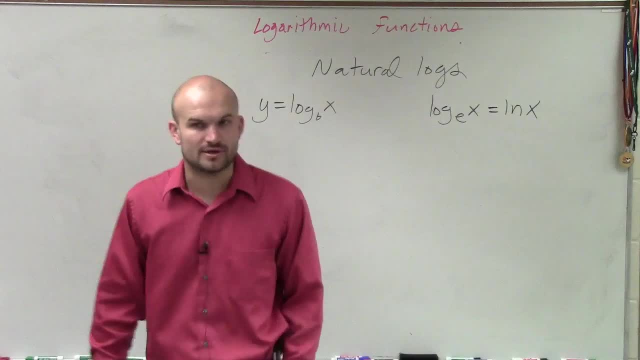 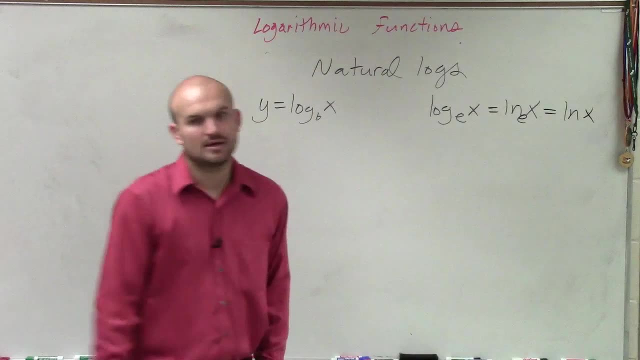 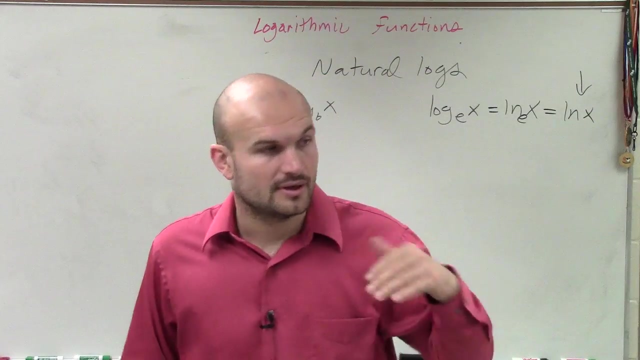 we see that ln of x, which is just a natural logarithm, and a natural logarithm still has a base e. Okay, But here is the form that you guys are going to see it in. So if I take a logarithm and I write it with a base e, we write that what that really means is ln. 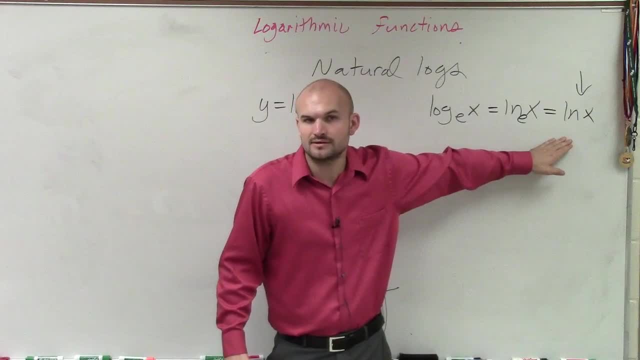 base e of x, which is really just ln of x. Okay, So that all when I, if you see an equation, you know you're going to ask me: what does that mean? It's because it's a base e of x. 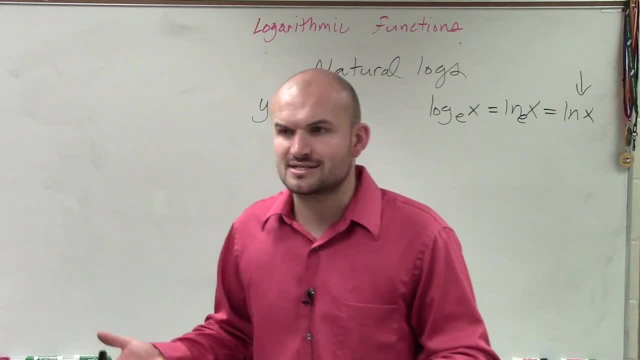 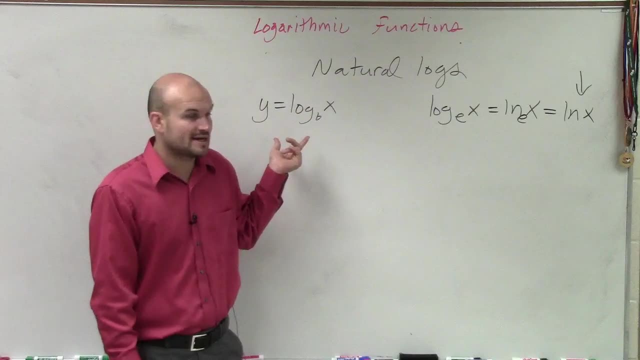 And if you see an equation or a problem and you say, oh, it's ln of x. well, what does ln of x represent? All it represents is a logarithm, a common logarithm with a base e. So it's the exact same thing. 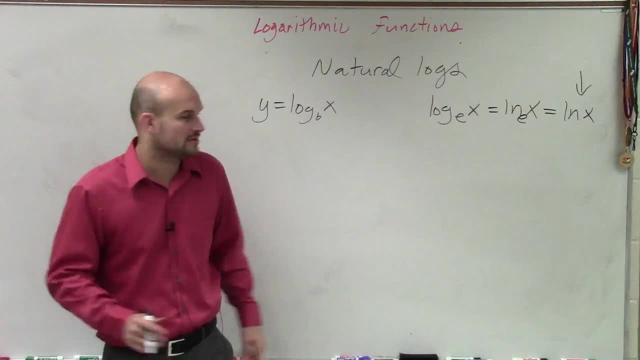 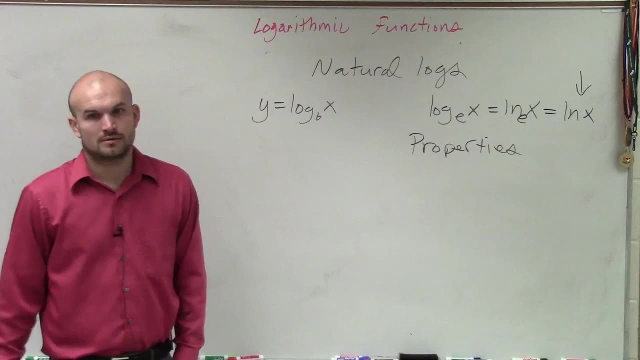 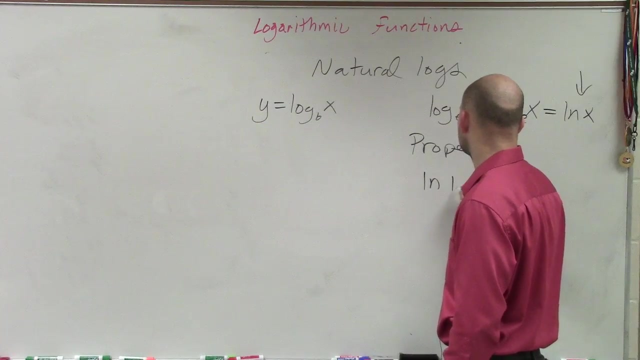 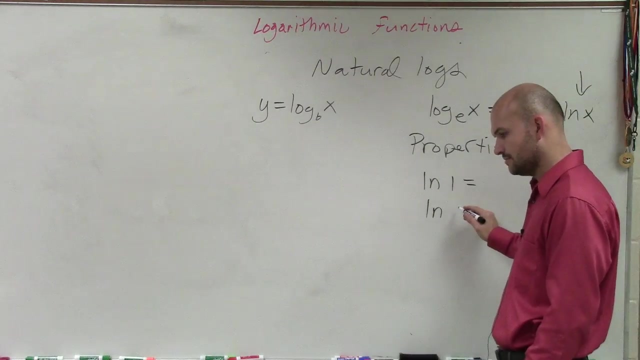 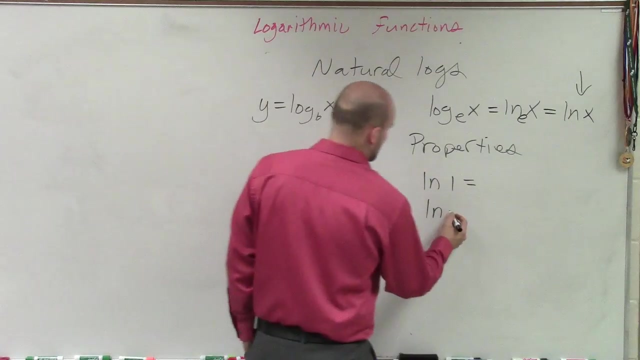 It just means the base is e instead of an integer. So when we talk about the properties, if you have ln of 1, ln of, was it e raised to what power equals 1?? Oh, ln of e, ln of e to the power of 1.. 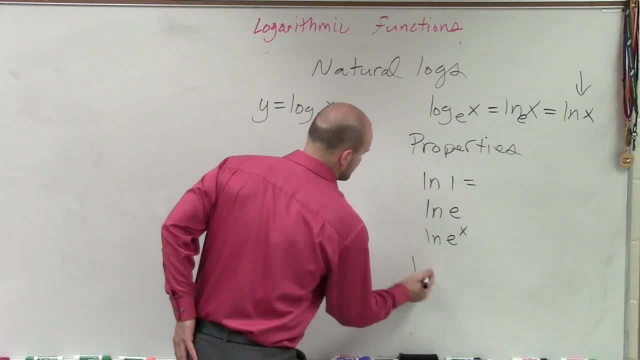 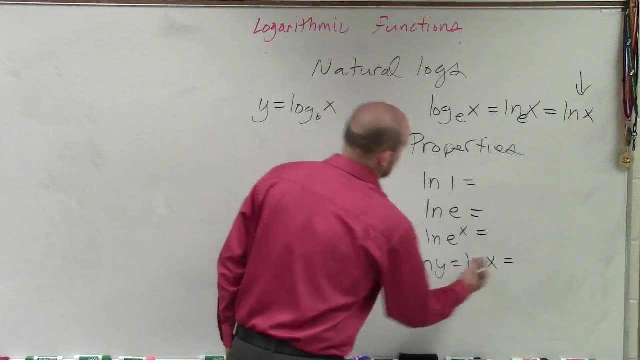 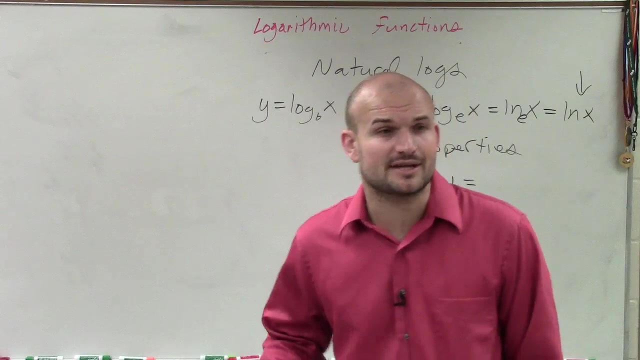 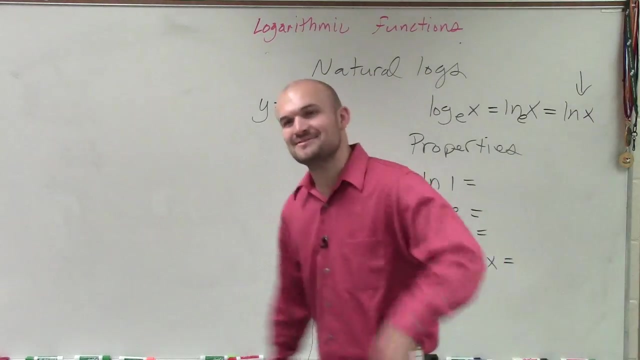 ln of e to the x And then you have. So, by going through these problems, what again I can do is I can go back, Marissa, and I can check. I'm sorry, Oh, OK, I'm just making sure. 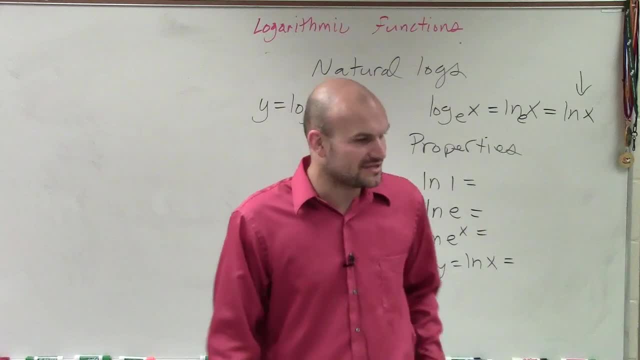 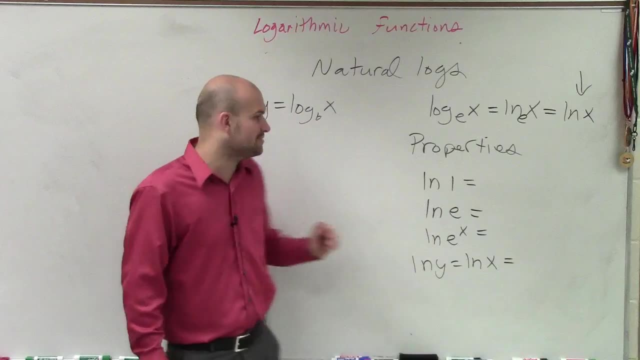 So now what we can do is, again, we can go back to converting by using our form. So again, what we can do is we can transfer each one of these to exponential form to see what it'd make. So if I transfer this, remember I said ln that has a base e. 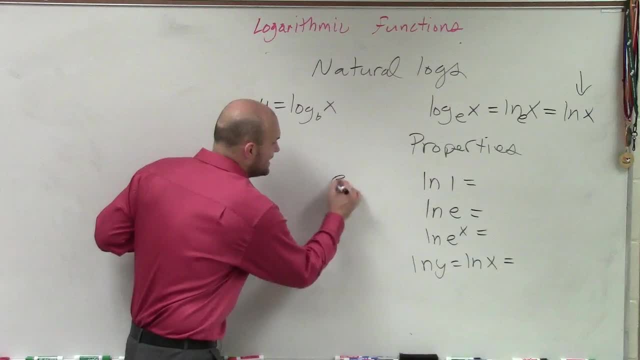 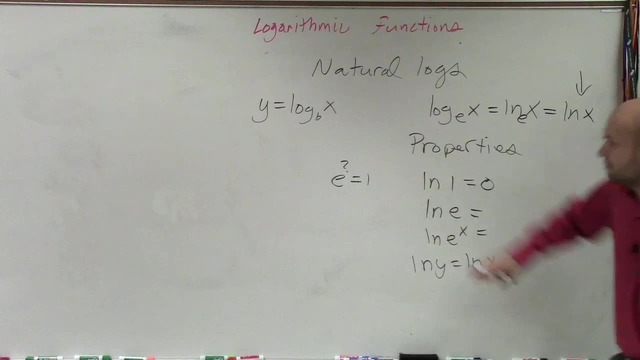 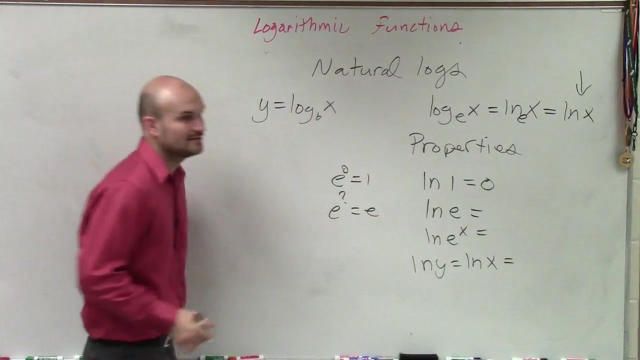 ln has a base e. So I can say: e raised to what number equals 1? 0. So ln of 1 equals 0. This has to be 0.. e raised to what number equals e 1. 1.